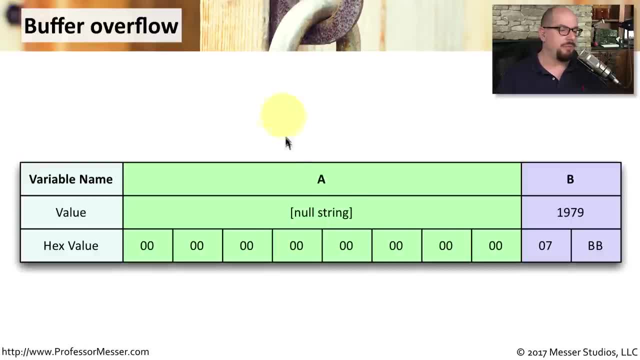 Here's an example of a buffer overflow. This is an application that has been written to contain two different variables- It's variable A and variable B- And you can see there has been some space allocated for each variable. You can see that variable A has one, two, three, four, five. 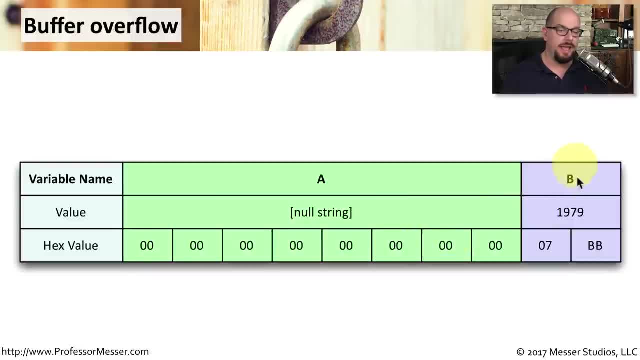 six, seven, eight bytes that it can use to allocate information And you can see that variable B has two bytes available. There's already information that has been saved into variable B. You can see the value is 1979.. If we look at the hex value it's 0, 7, bravo, bravo. 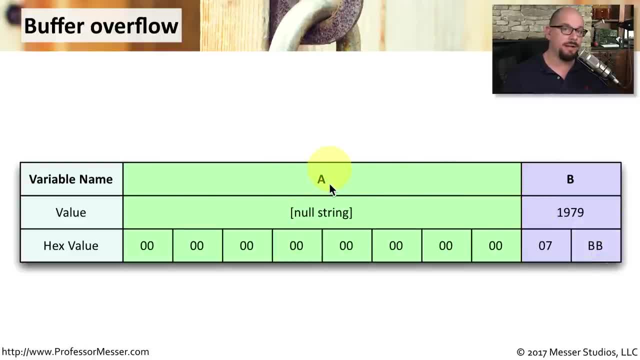 But the bad guys have realized the developer's not performing a bounds check for A, And not only can you write eight bytes into A, you can write more than eight bytes, causing a buffer overflow. So the bad guys will write into variable A nine bytes of information. 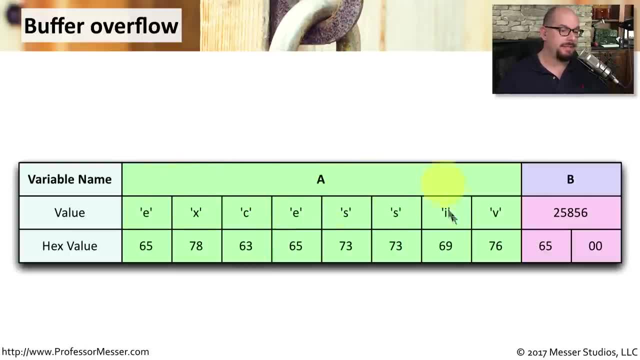 And you can see that it takes E-X-C-E-S-S-I-V, And then they actually put an E on the end And that E is written into the first byte of variable B, something that should not happen if you're writing information to a single variable. 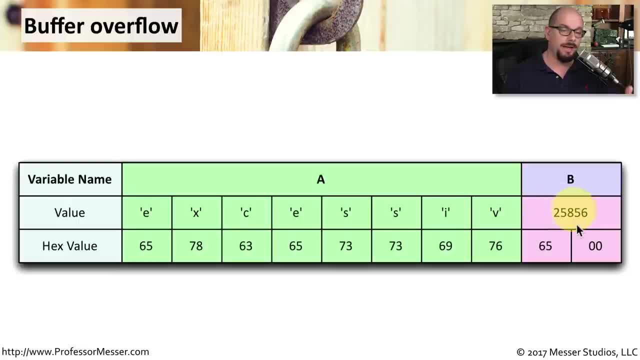 This is now changed, Variable B to be the value 25, 856.. Very different than the original variable. That obviously is something that should not have happened. You should not be able to write information into variable A and have it change something in variable B. 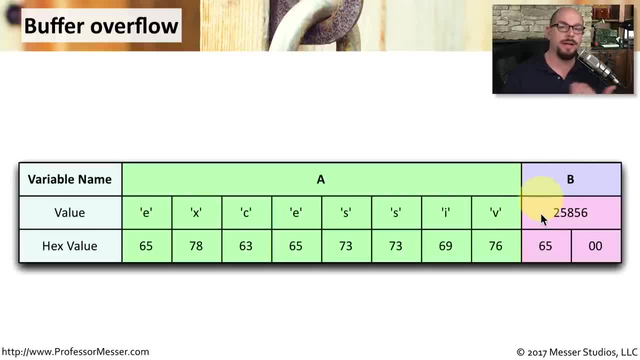 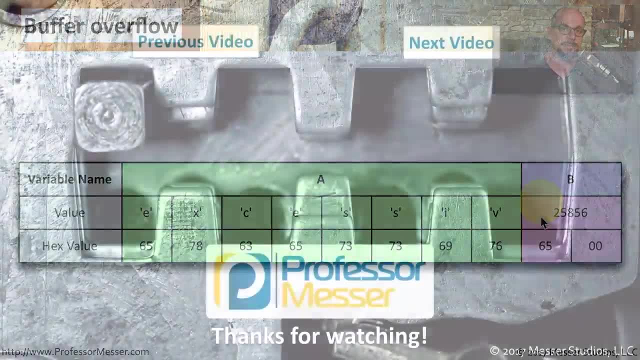 Now the bad guys will be able to take advantage of this. They'll try writing different things into variable B and see if that provides them with an access that they would not normally have into your system. That's why I'm saying I spoke about how simple that is. 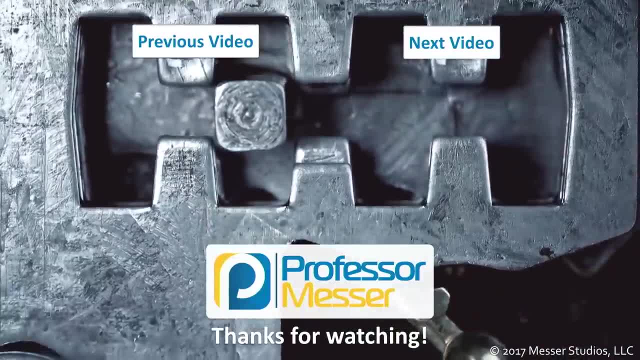 and it's probably a little bit confusing for two people. It's a little bit difficult to talk about this in a way. that's definitely not easy to do, But if you can run it in an easy way, I mean if you can run it a little bit faster. and then you just give it that one week. it should be a little bit easier to replicate. You should not be able to write anything into variable A, into variable B, or even want to go back and do a final piece in variable A or something like that. Because if you're writing something into variable B, 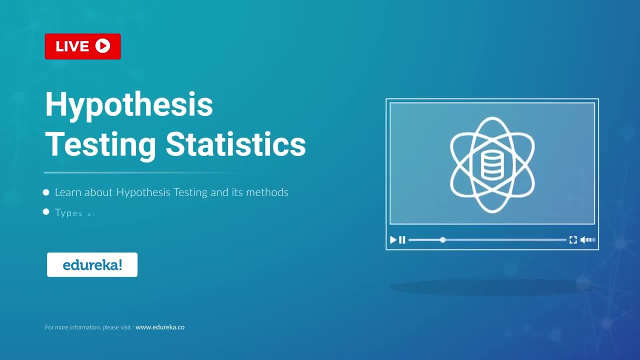 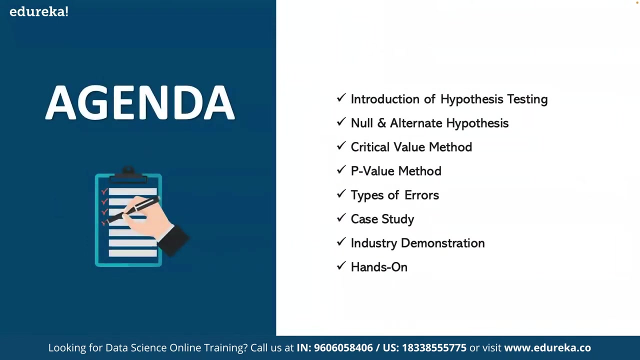 Hey everyone, thank you so much for joining in So as we progress. in today's session we'll be learning the statistical hypothesis testing, So we'll look into what exactly is this hypothesis testing. We'll understand about the concept of null hypothesis and the